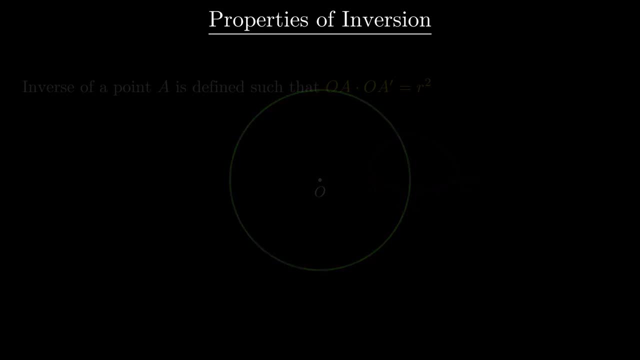 OA. Inverse of a line passing through the center of inversion is the same line. It doesn't change. Inverse of a line not passing through the center of inversion will always be a circle passing through the center of inversion. Inverse of a circle not passing through the center of inversion is a circle. 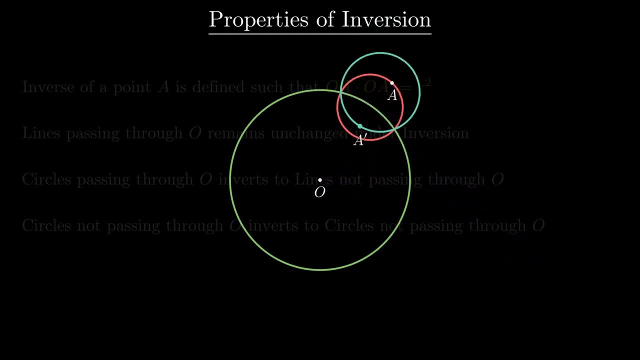 not passing through the center of inversion. Circles orthogonal to the inversion circle remain invariant under inversion. The angle through which two curves intersect does not change under inversion. This property is very useful because it tells us that the number of intersection points and tangency points remain the same under inversion. 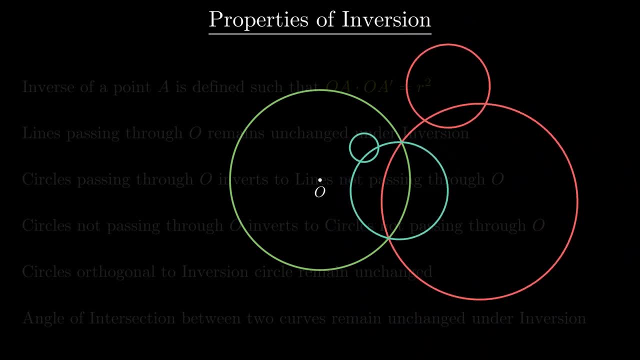 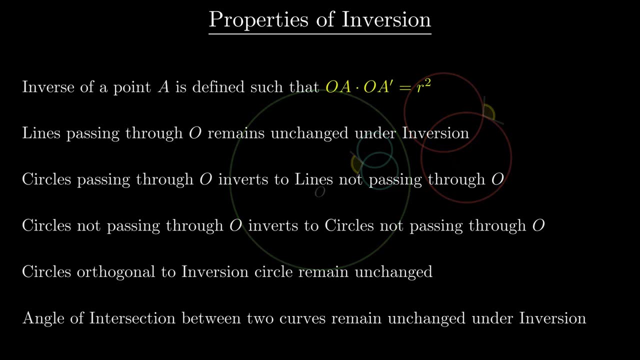 That is a lot of information, So now we shall discuss about the angle, which doesn't change under inversion. The number of intersection points and tangency points either remains the same under inversion, So now is probably a right time to pause the video and take a closer look at these properties. 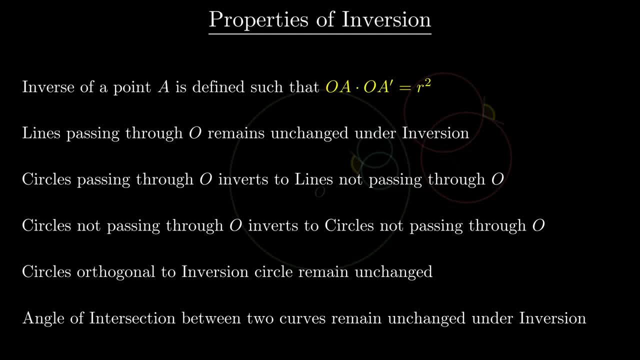 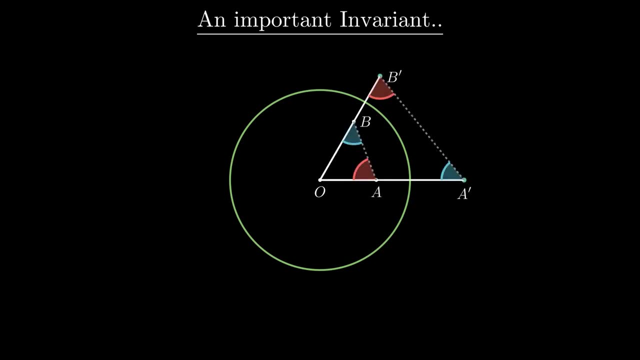 Quite amazingly, all of these properties can be proved with just basic geometry. You can always visit the paper strain video where we have proved all this. Before proceeding with the solution, we revisit something very important. We can easily see that circle inversion alters the distance between any two points. 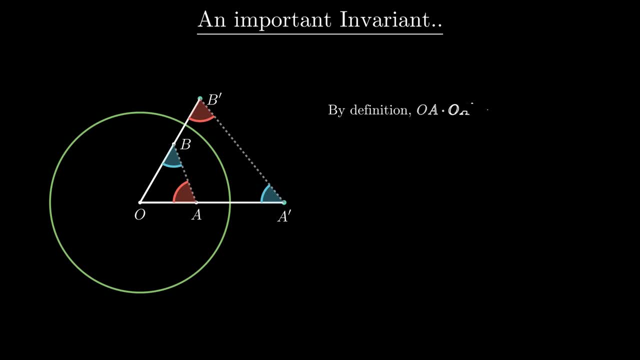 This variation in distance can be quantified using the idea of similar triangles. Simply put, the distance between points A and B before and after inversion can be related by the expression A dash. B dash equals AB times R square by OA times OB. One of the key properties that makes inversion such a powerful tool is the idea of cross ratio. 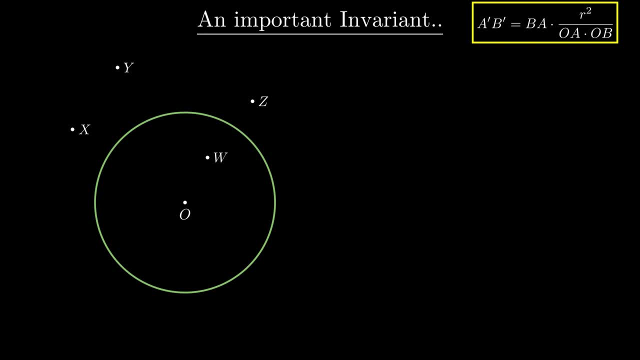 Given any four points: W, X, Y and Z. the cross ratio is defined as a product of the ratios W- X by W- Y and Y Z by X- Z. This is usually denoted by the Greek letter lambda. We can prove its invariance easily using the expression we had for the distance between two points. 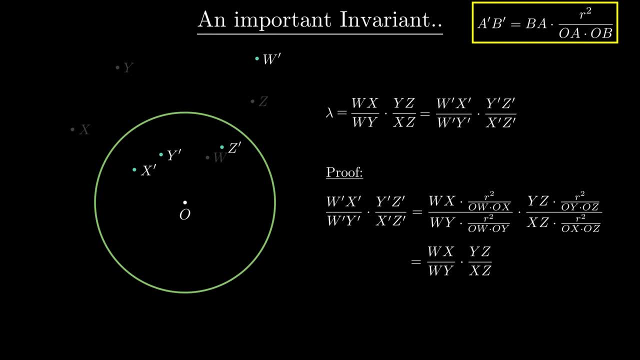 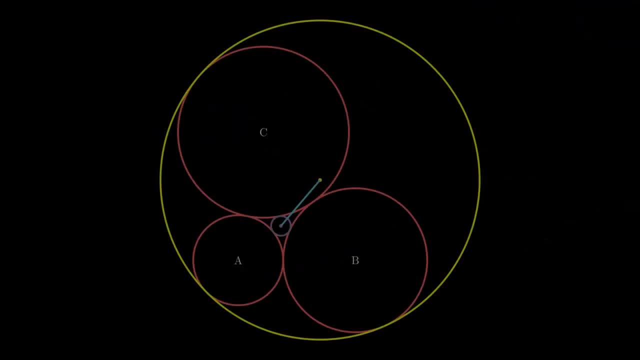 Just make the usual substitutions and a bunch of cancellations. later the equality becomes apparent. Consider these four points in our problem. Let capital R be the radius of the circumscribing circle, small r be the radius of the inscribed circle and d be the distance between their centers. 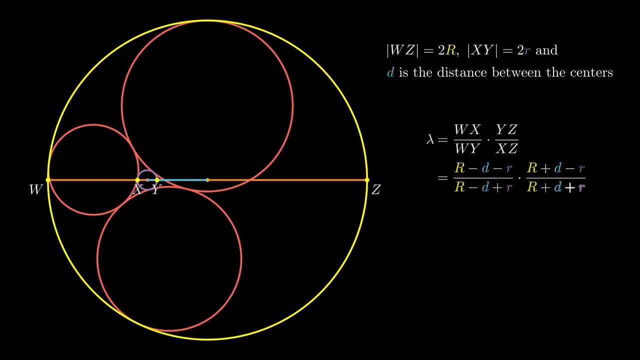 Now the cross ratio between these points can be expressed in terms of the radii of these quantities quite easily. The terms in the cross ratio are obvious from the geometry of the circles, and we arrive at this expression for the cross ratio. Our plan to solve the problem now is to make a clever choice of inversion. 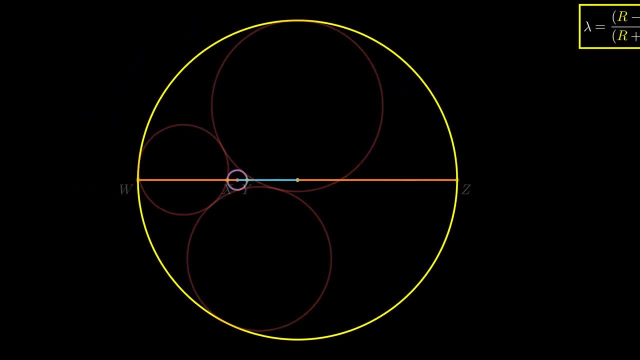 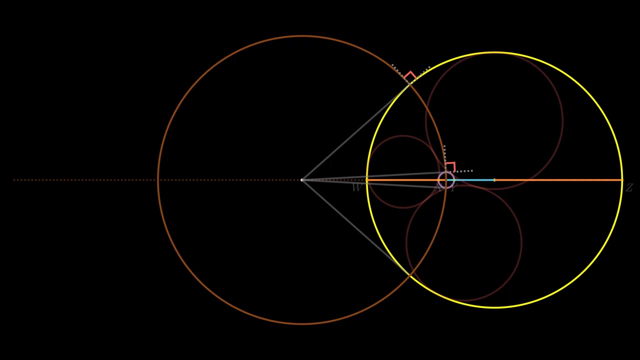 And use the invariance of cross ratio to simplify the problem considerably. We begin by constructing a circle that is simultaneously orthogonal and collinear to both the circles. By orthogonal, we mean the brown circle intersects, the circumscribing and the inscribed circles at right angles. 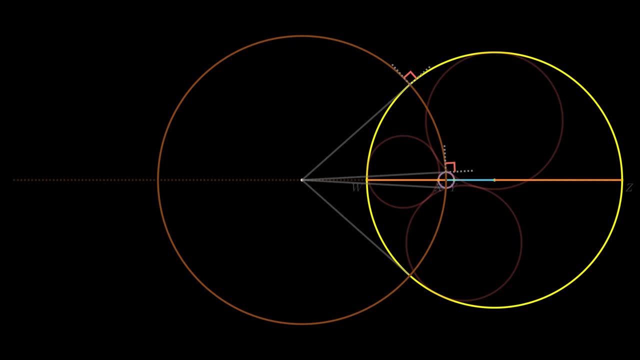 Here's a small challenge. Can you see how we can find a circle simultaneously orthogonal to two given circles? If you can share it with us in the comment section below. Now take this point: the point of intersection between the orthogonal circle and the line of centers. 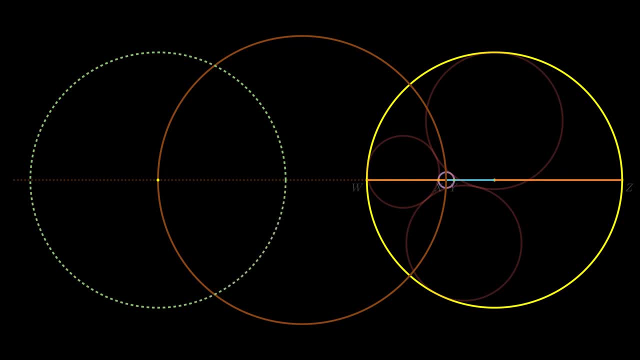 as the center of inversion, with some arbitrary radius of inversion. The radius of inversion actually is irrelevant, as can be seen shortly. Let's see what happens to our setup with this choice of inversion. The line of centers passes through the center of inversion. 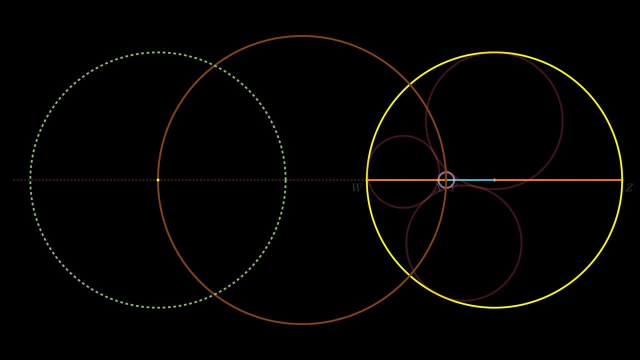 so it remains invariant. The orthogonal circle passes through the center of inversion and is perpendicular to the line of centers. Its inverse then becomes a straight line perpendicular to the line of centers. The yellow circle is perpendicular to both the orthogonal circle and the line of centers. 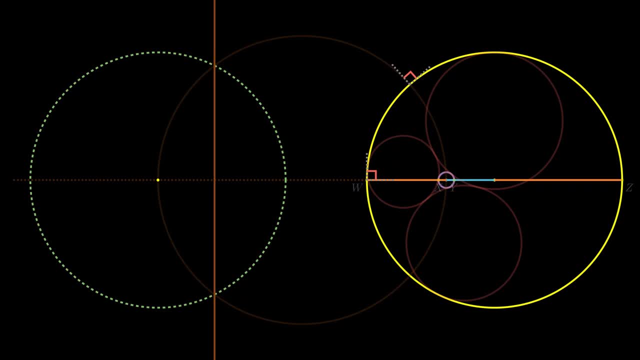 Hence its inverse, which is a circle, will also be perpendicular to both the line of centers and the orthogonal line. That is only possible when the inverse of the yellow circle is symmetrical to both these lines. The same applies for the other circle as well.